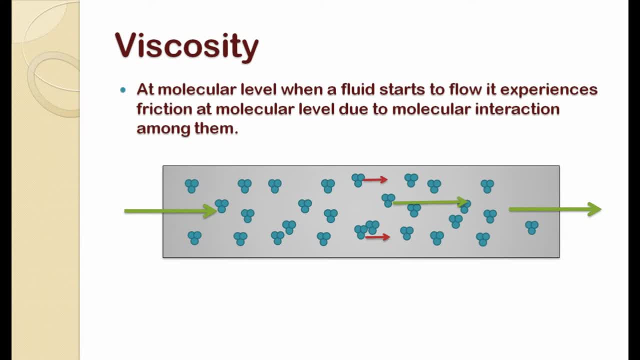 more velocity than layers of fluid or molecules which are close to the inner surface of tube. Due to this difference in velocities of fluid layers, the layers with low velocity are more resistant to the flow of layers with high velocity, And if the intermolecular resistance 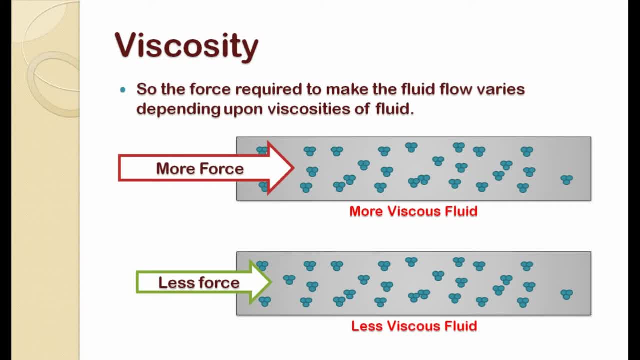 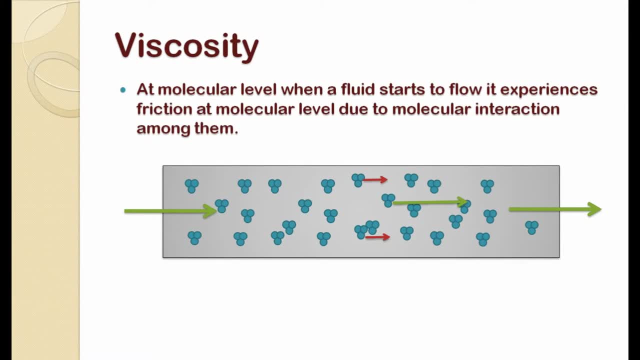 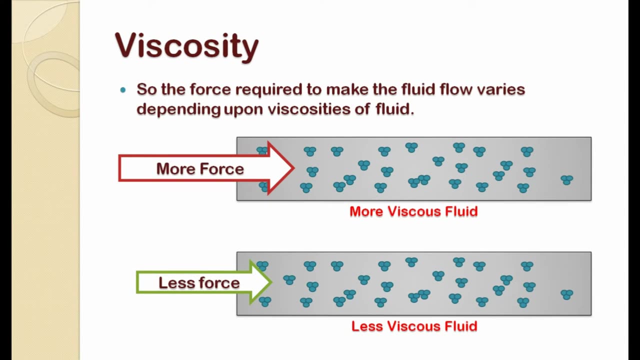 is very high, then overall speed of fluid flow decreases. Such fluids with high resistance to flow are called as viscous fluids. In short, if we want the fluid to move, we have to apply the force so as to overcome this resistance. If the fluid is more viscous, we have to apply 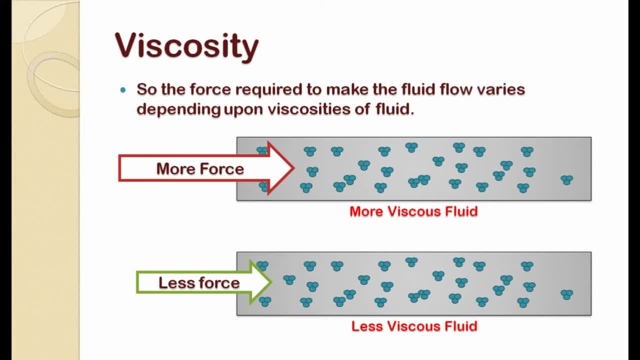 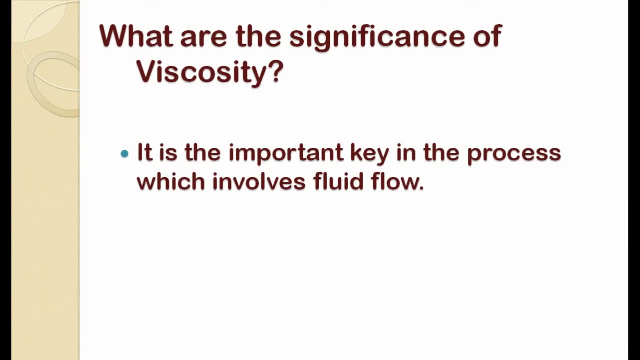 more force, Whereas if the fluid is less viscous, then resistance will be less and the force required will also be less. Term viscosity is very important term of fluid mechanics. Wherever fluid flow occurs, we have to take the viscosity into consideration. 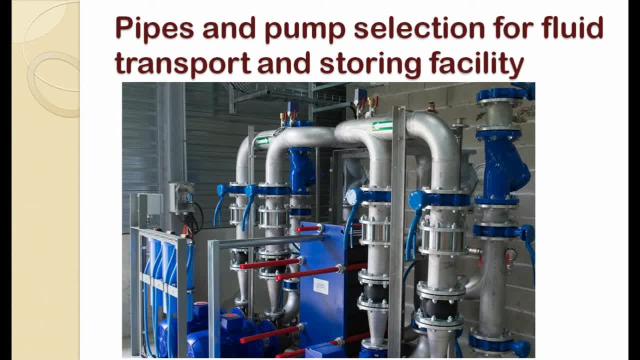 During design process of any fluid carrying or storing facility, we have to take the viscosity into consideration. Selection of pumps, pipes and other accessories mainly depends on viscosity of fluid. If we are designing a system for slurry handling, the pipes and pumps will be different than 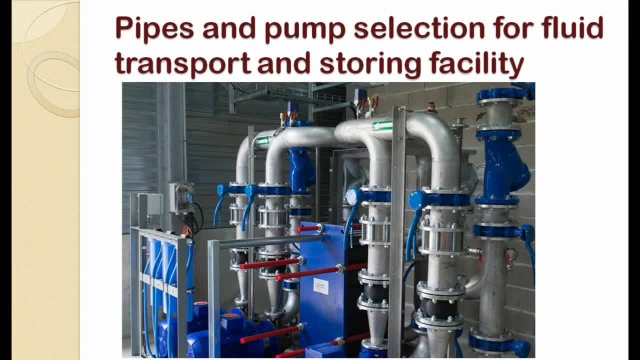 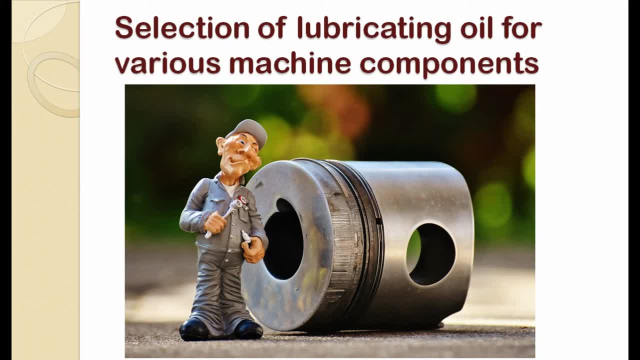 the system which is designed to carry water or oil. Now the next example is selection of fluid. The first method of selection is the application of lubricant. It also depends upon viscosity of fluid. While selecting the fluid for lubrication purpose, it is expected that the fluid should. 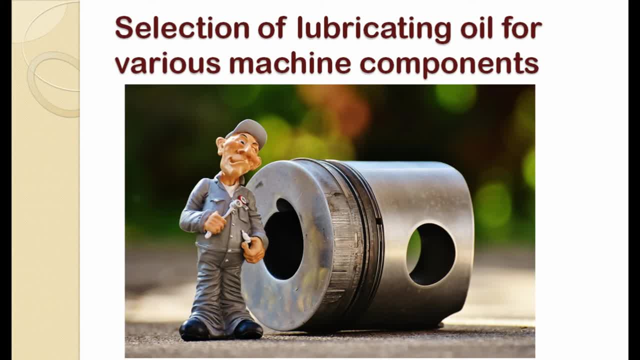 also, It should always maintain a constant film of oil due to moving fast, so as to avoid friction and allow smooth motion. but same time it is expected that it should not create any resistance to the motion. Here also, viscosity is the important criteria, which helps us in selecting. 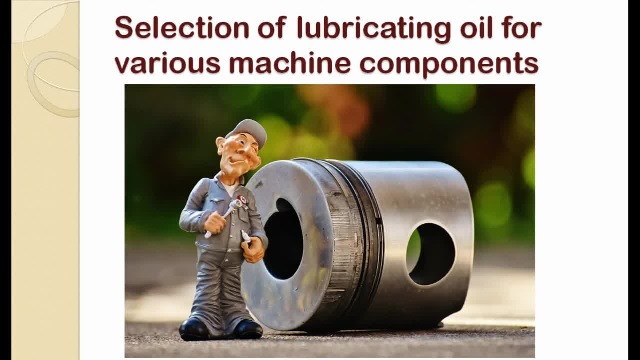 correct lubricant. So, friends, I hope you have understood the topic well, but still, if you have any doubts, please comment below. Thank you for watching.